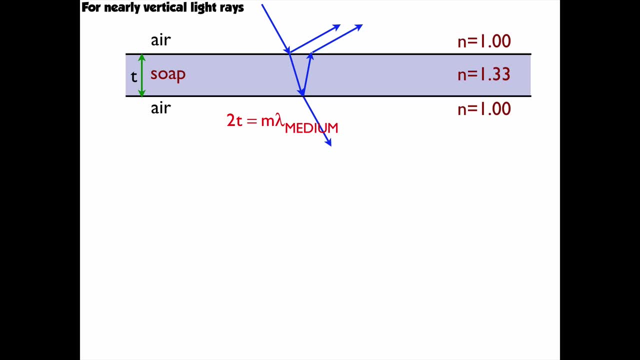 so I know that that's the path length difference. Twice, the thickness is equal to M lambda, which is the path length difference. But notice that because the path length is in the film and not in the air or the vacuum, the wavelength is going to differ, and that's what's important. 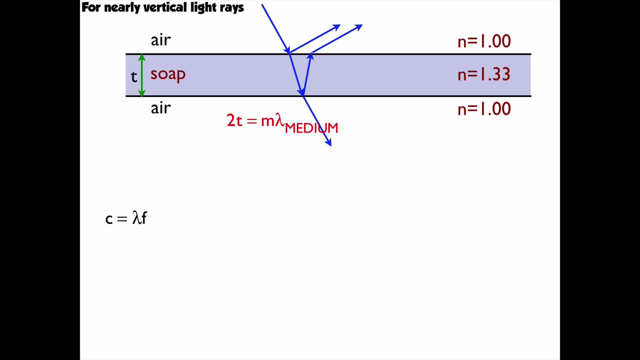 So I need to account for that. So I use the wave equation. C equals lambda F and the index of refraction is C over the velocity in the medium, which means that the wavelength in the vacuum or air is the same. 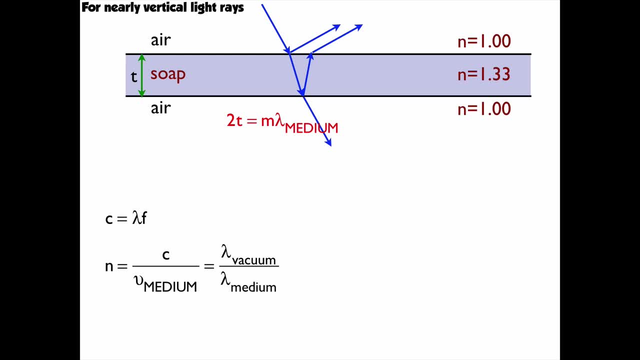 Divided by the wavelength in the medium, is equal to the index of refraction. When I rearrange that the wavelength in the medium is equal to the wavelength in the vacuum, which is the same as air divided by the index of refraction, 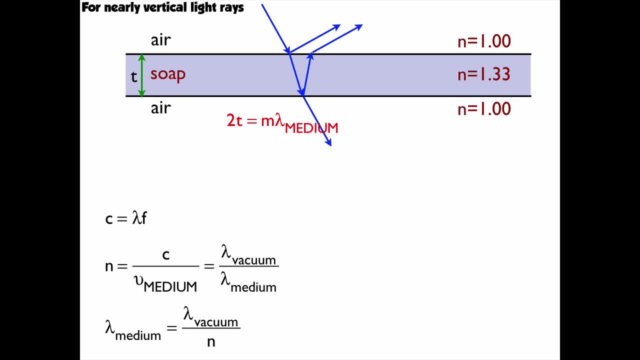 Now I've got one more little hitch to this. Whenever a light ray goes from a low index to a high index, like from air to soap, I get a 180 degree phase change or lambda over 2 phase change. Whenever a wave goes from a high index to a low, the opposite, that's. 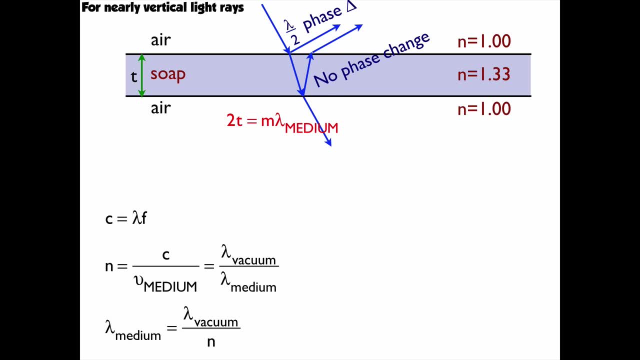 when I don't get a phase change, There's no phase change there. So because it's a phase change, usually we know when the path length is equal to m lambda, I get constructive interference, I get a bright spot. But here, because that lambda over 2 phase length, instead of a bright 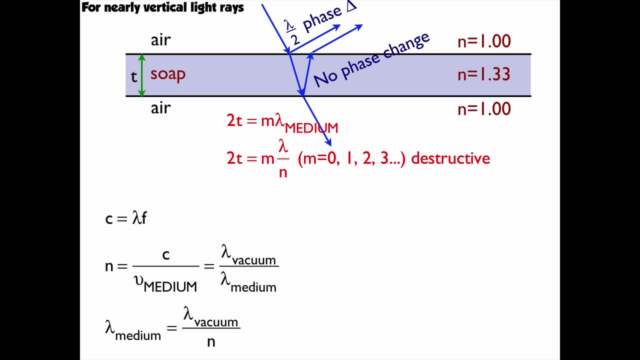 spot, I get a dark spot. In other words, I get destructive interference. So twice the thickness is equal to m lambda over n, and my orders are 0,, 1,, 2,, 3, and that's destructive. So these are the frequencies that it's blocking out And the frequencies that you see constructive. 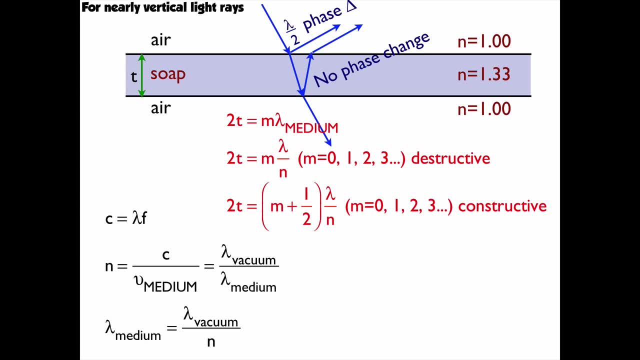 interference would therefore be m plus. Now, just so you know, there is an alternative format of writing this equation: You can multiply both sides by the index of refraction and you get 2 nt is equal to m lambda and 2 nt. 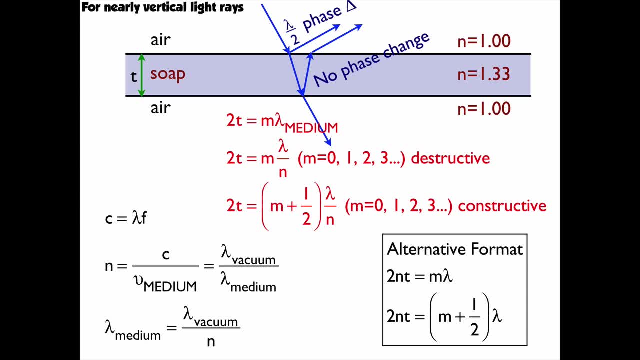 is equal to m plus a half lambda. But to me, this equation really doesn't tell the story of the fact that you have to change the wavelength in the substance, which is why it's lambda over m. Okay, let's look at a different situation, And this time I've got glass on the bottom. 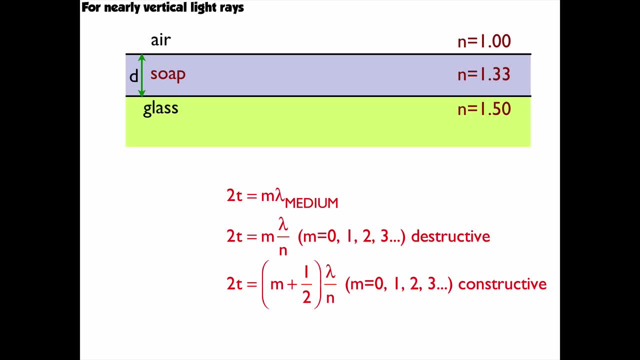 sorry, I've got air soap sitting on top of glass And you can see how my indices of refraction have changed. So this is the equation that we had before: The light comes in, reflects and refracts, then reflects and refracts all the way down. And I'm going to ignore.